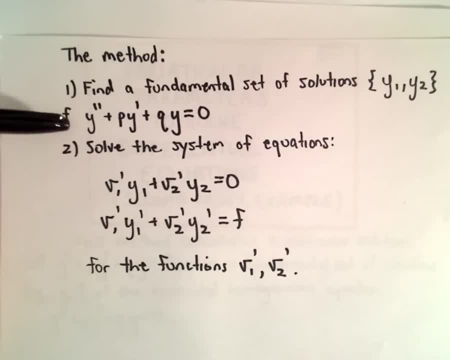 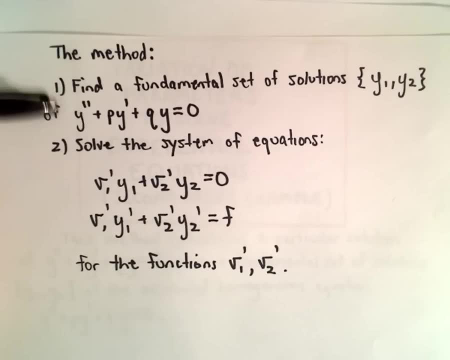 We can use reduction of order to find the other, and I've definitely done examples about reduction of order, about how you go about finding that second example, given the first one. So, okay, in my example, the first example I'm going to do, at least we're going to be given the fundamental set of solutions for free. 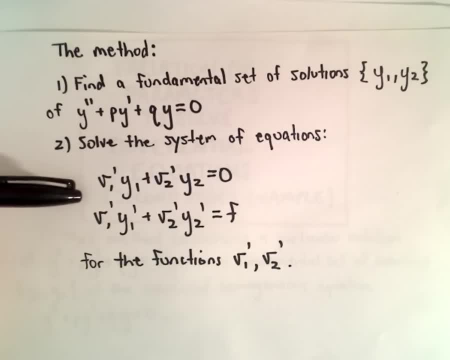 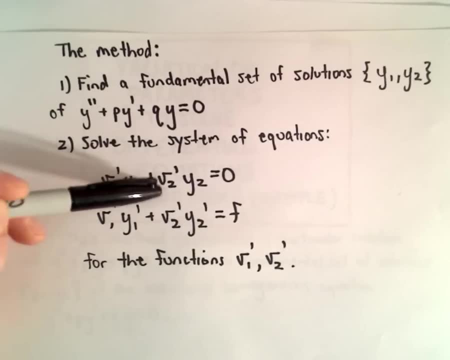 Okay. so after that, to me it seems relatively straightforward, at least in this second order case. What we do is we solve the system of equations v 1 prime times y 1, plus v 2 prime times y 2. We set that equal to 0.. 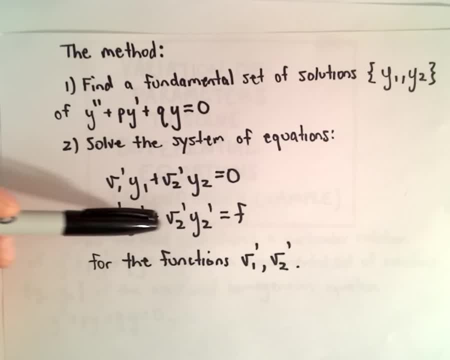 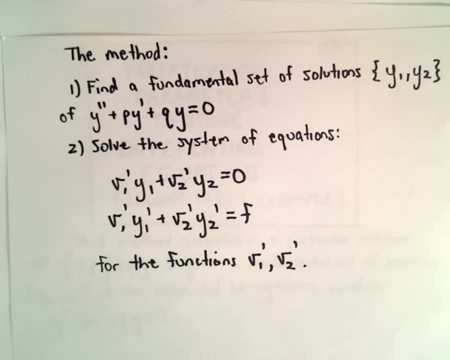 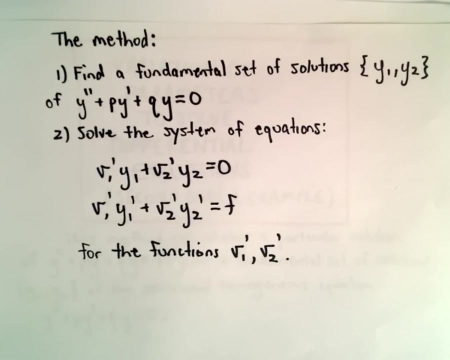 Then our other equation: v 1 prime times y 1 prime plus v 2 prime times y 2 prime equals f. We're going to solve that for the functions v 1 prime, v 2 prime. Once we have those, we'll calculate an antiderivative and that's going to help us come up with our particular solution and also our general solution. 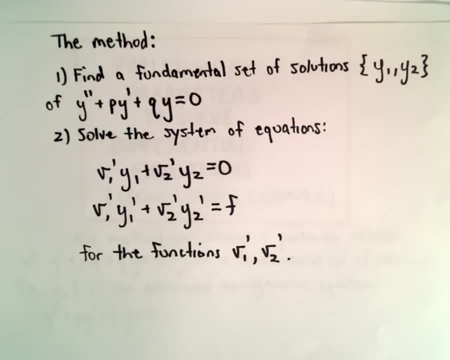 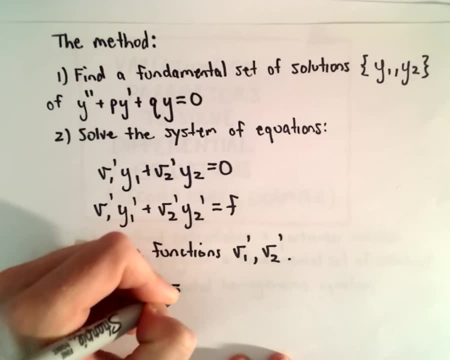 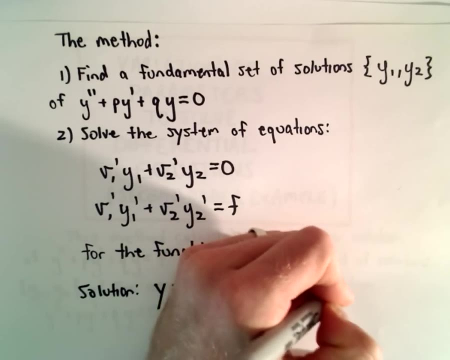 So I should say somewhere I left this out. Once we have that, our solution is going to look like: y equals v 1 times y 1 plus v 2 times y 2.. This is going to be a particular solution. 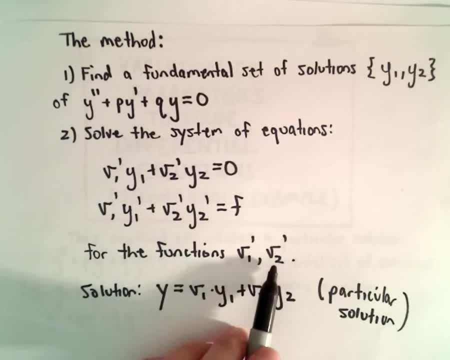 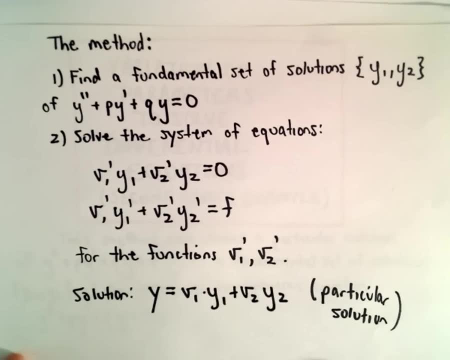 Okay, so that's going to be the idea. So once we figure out v 1 prime, v 2 prime, we can figure out v 1 and v 2, multiply that by the original fundamental set and that's going to give us a particular solution. 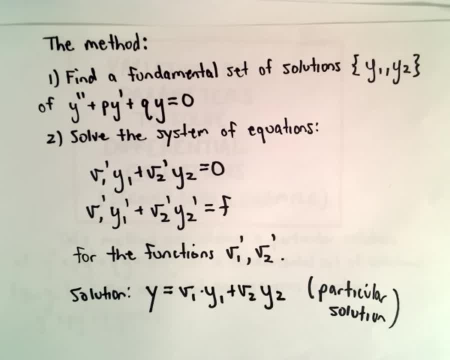 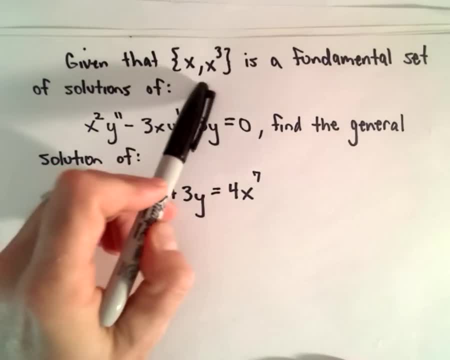 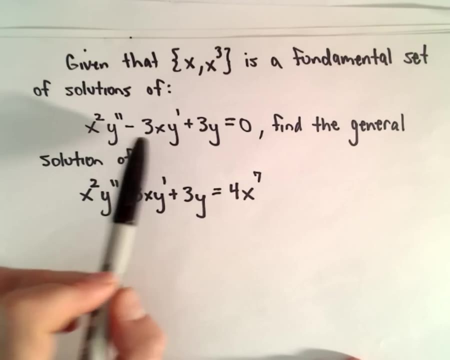 So that's why we're interested in finding v 1 and v 2.. Alrighty, so let's do an example here. So suppose that we're already given again for free that x and x to the 3rd. that is a fundamental set of solutions to the equation: x squared times y, double prime minus 3x times y, prime plus 3y equals 0.. 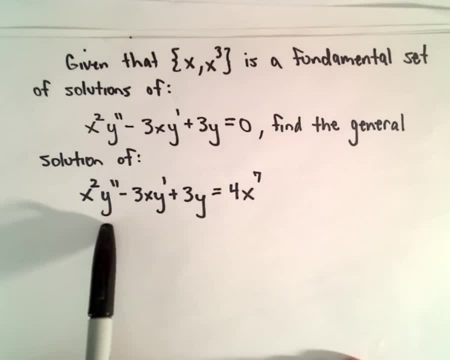 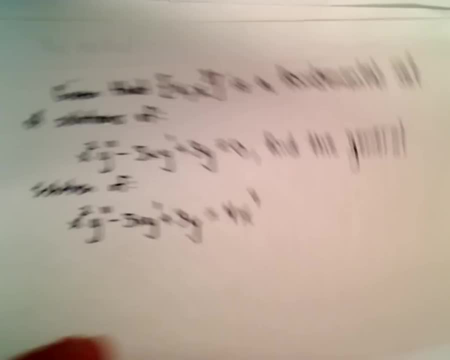 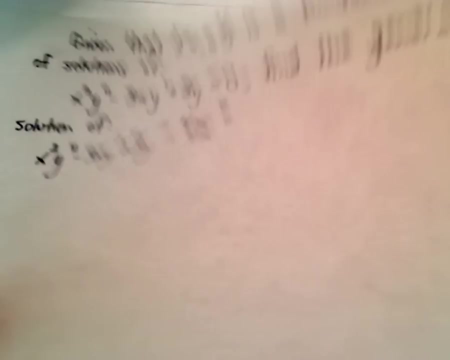 We're going to find the general solution of x squared times y double prime minus 3xy. prime plus 3y equals 4x to the 7th. Alright, so The first thing I'm going to do is sort of put this into the correct form that I want. and the form that we want is we want just y double prime at the beginning. 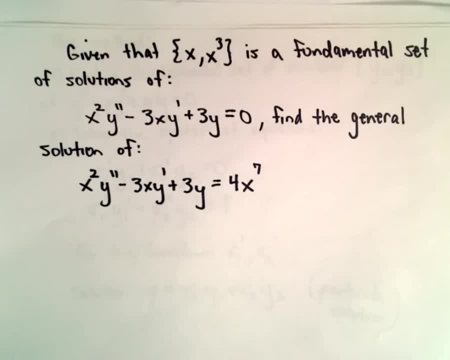 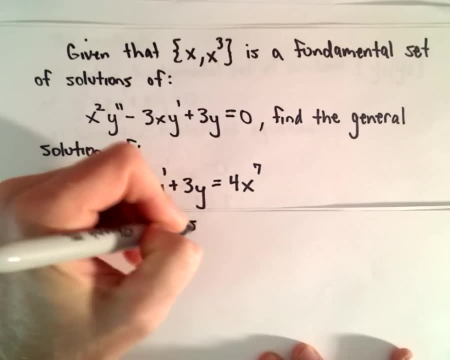 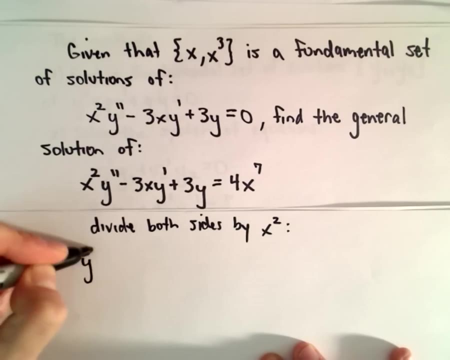 We don't want this function of x hanging out front. So all I'm going to do to get started is just divide both sides. I'm going to divide both sides, in this case, by x squared. So if we do that, we'll be left with y double prime. 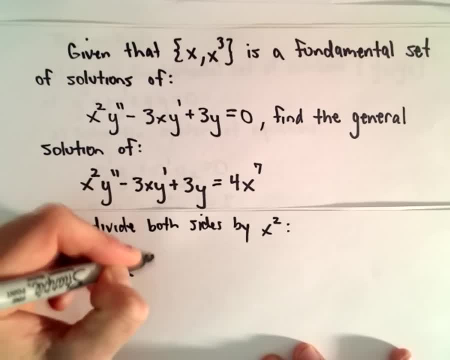 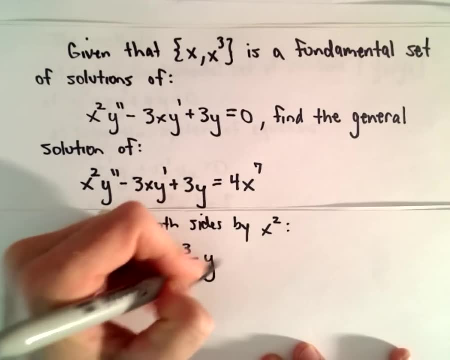 3x divided by x, x squared, that's going to leave us with 3 over x again times y prime. Well, 3 divided by x squared is 3 divided by x squared, multiplied by y. And then 4x to the 7th divided by x squared, that'll simply be 4x to the 5th power. 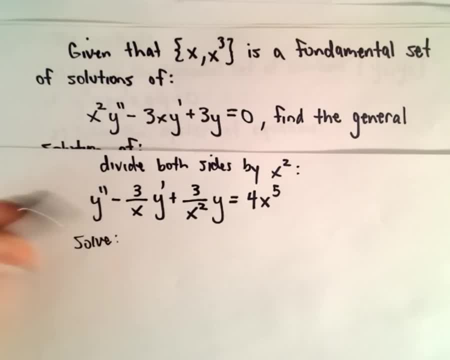 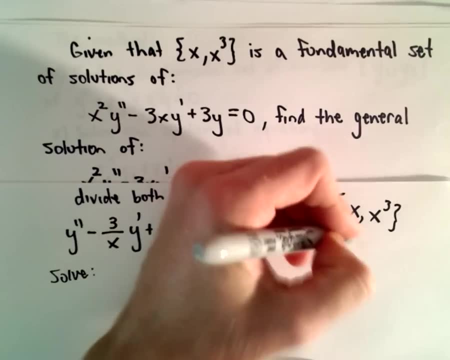 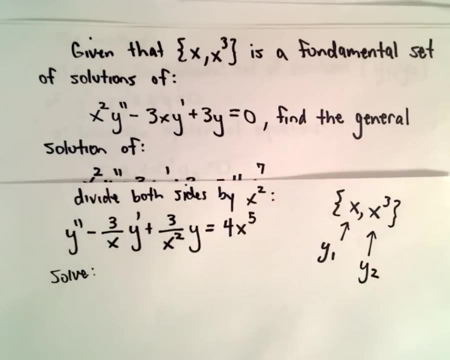 Alright. so now we have to solve our system. So we have to solve our system. So again, x and x to the 3rd. those were our fundamental set of solutions. So I'm going to denote x is our y sub 1, and I'm going to denote x to the 3rd as our y sub 2.. 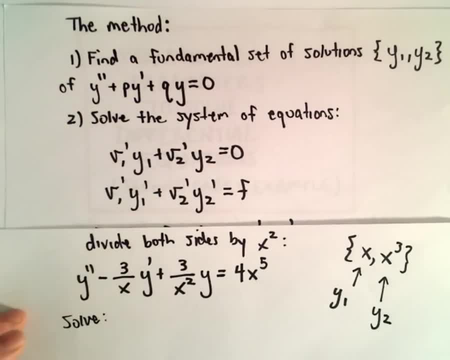 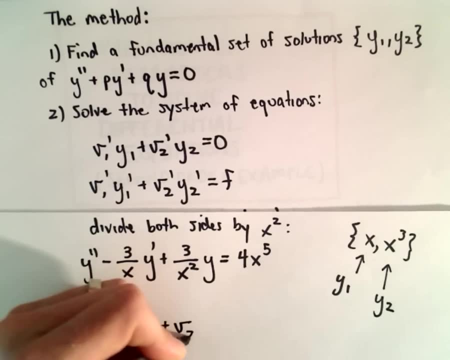 And now all I'm going to do is just look at this system of equations. That's what we're going to have to solve. So we've got v1 prime times y1, which is x, plus v2 prime times y2, which is going to be x to the 3rd. 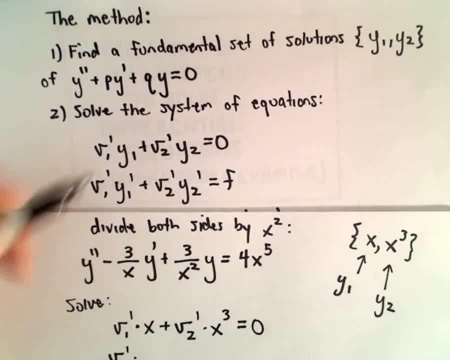 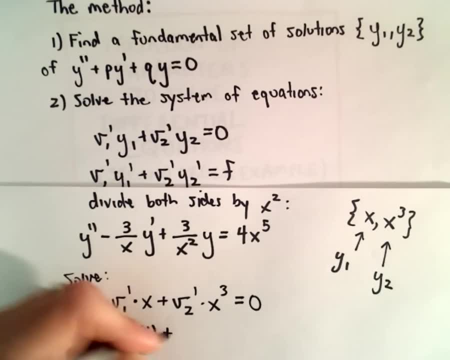 And then the other equation will be v1 prime. and then it says: take the derivative of our y1, so the derivative of x here is simply going to be 1.. And then we have plus v2 prime. Then we do the same thing. 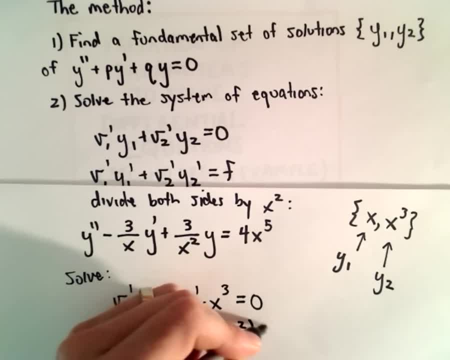 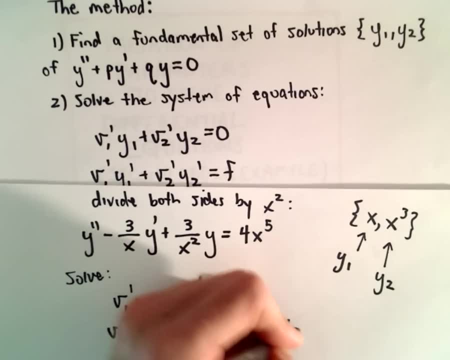 We take the derivative of x to the 3rd, which is going to be 3x squared, And then, on the right side, we use our function f, which in this case is going to be 4x to the 5th power. 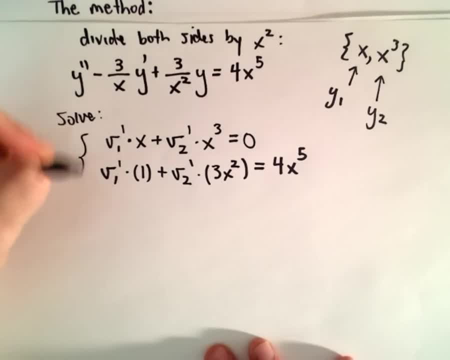 So now all we have to do is solve this system of equations. So I'm going to solve this using substitution. So I'm going to solve this using substitution. So I'm going to solve this using substitution. Feel free to solve it any way you want. 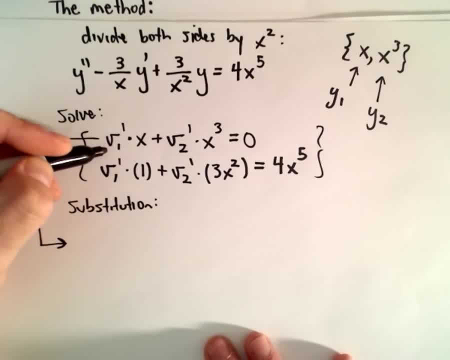 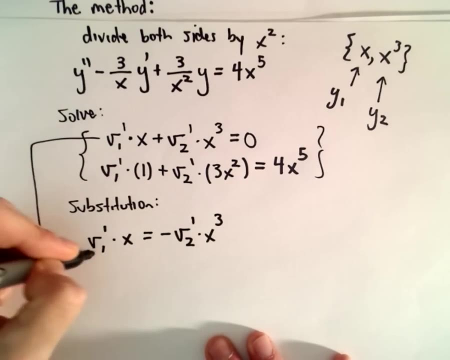 So if we take our first equation, if we solve- I just solved this, for what did I solve it for Probably just v1 prime. So I've got v1 prime times x. We can subtract the other term, So v2 prime times x to the 3rd. 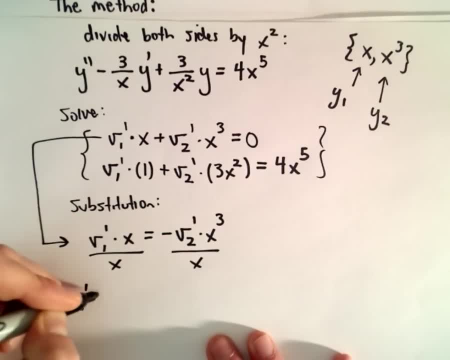 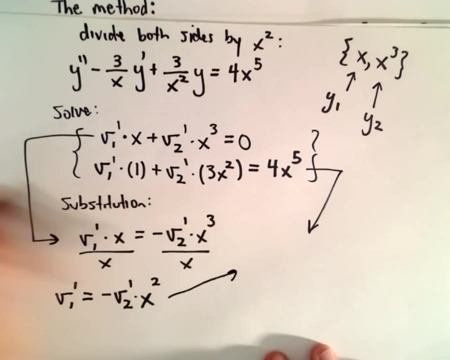 Well, if we divide both sides simply by x, we've got v1 prime equals. we'll have negative v2 prime, Then x to the 3rd. Well, hey, that's just x squared. Now all I'm going to do is just substitute that into our second equation. 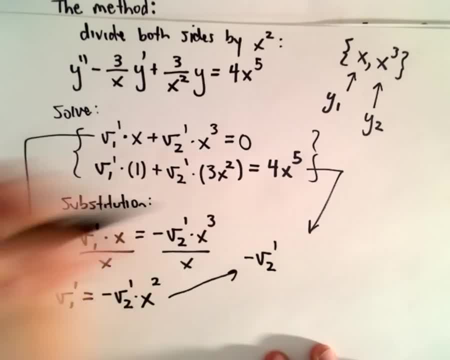 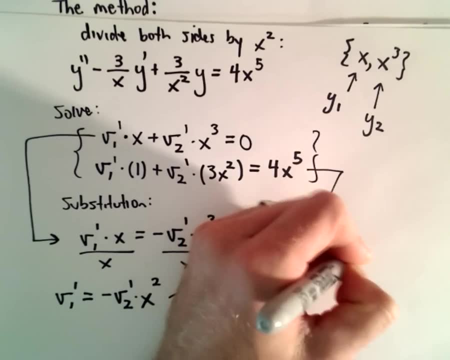 So v1 prime- that's going to be negative. v2 prime times x squared. Plus we've got again our v2 prime times 3x squared. That's going to equal 4x to the 5th power. 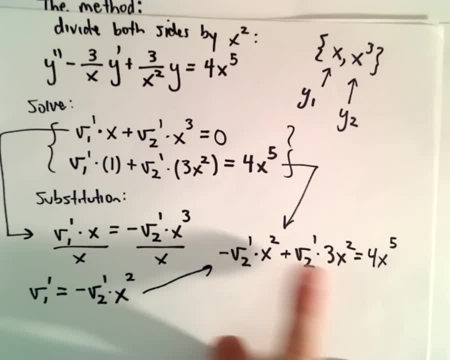 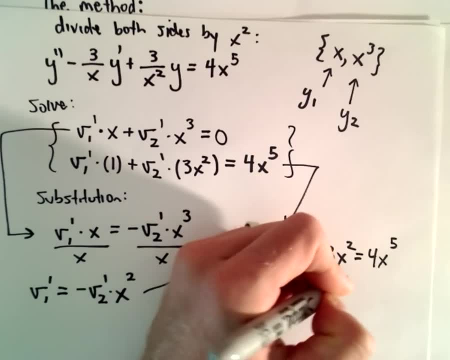 Okay. so if we combine our like terms, we've got negative x squared. We have a positive 3x squared. That's going to give us 2x squared times v2 prime. We have 4x to the 5th still hanging out on the right side. 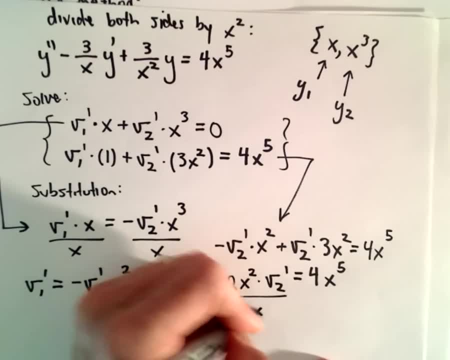 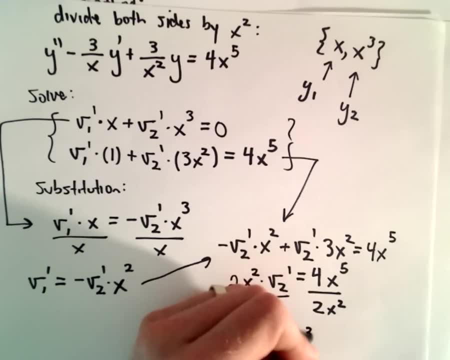 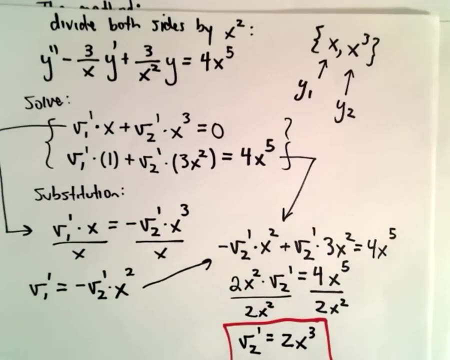 Well, we can just divide both sides by 2x squared, And now we're going to have that v2 prime equals 2 times x to the 3rd power. So that's already part of what we need. So now that we have that, 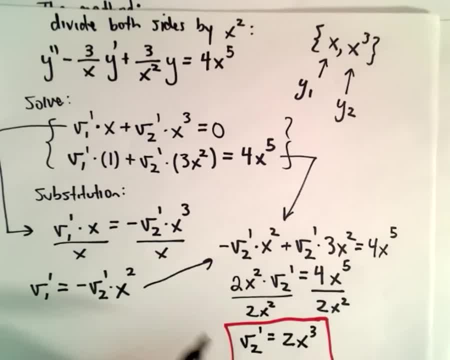 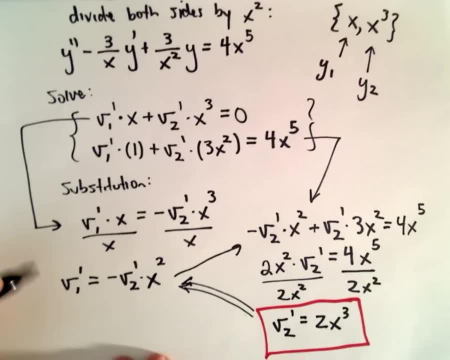 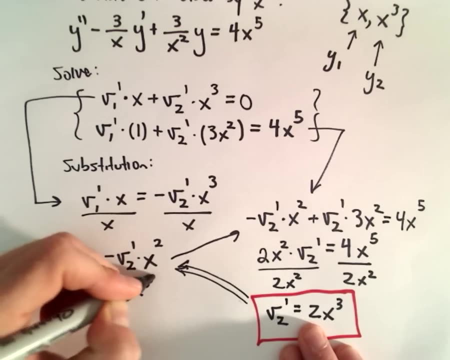 We can just go back and simply solve for v1 prime. So now I'm just going to substitute it back in here now. So that tells us that v1 prime is going to be negative. v2 prime, which is 2x to the 3rd. 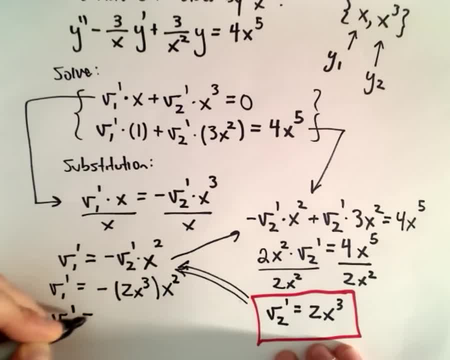 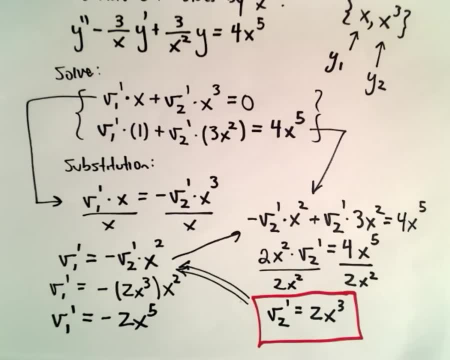 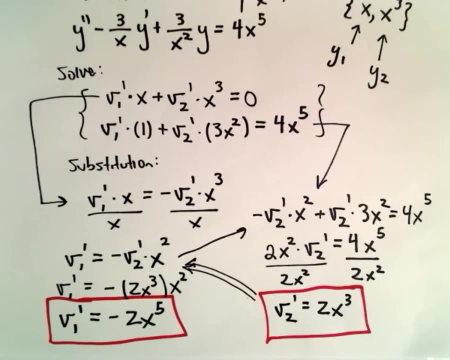 And then we multiply that by x squared, So it simply says that v1 prime is going to be negative 2x to the 5th power. Alright, so far, so good. And now we're almost there. We just have to calculate some antiderivatives. 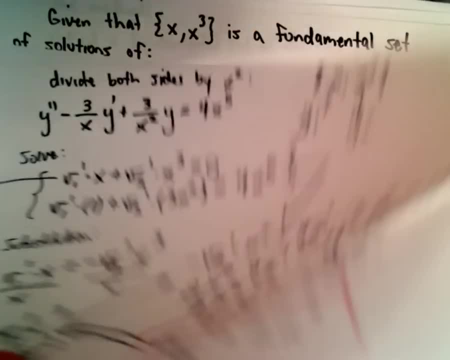 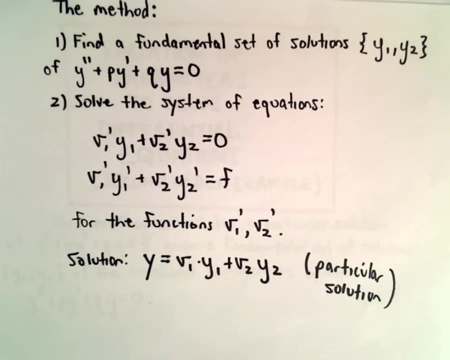 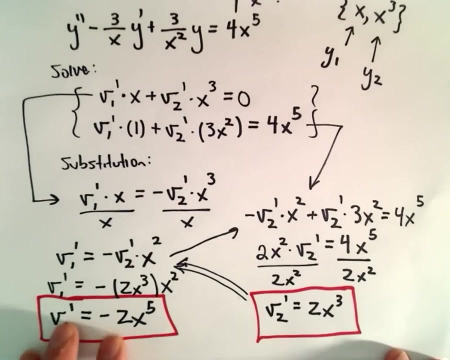 And to come up with a particular solution once we have the antiderivatives. we'll just calculate it using this bottom equation. Now, it's not always possible to come up with a nice, clean antiderivative. You know, these are very simple functions that we can integrate. 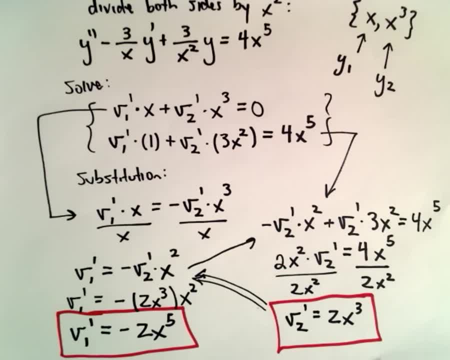 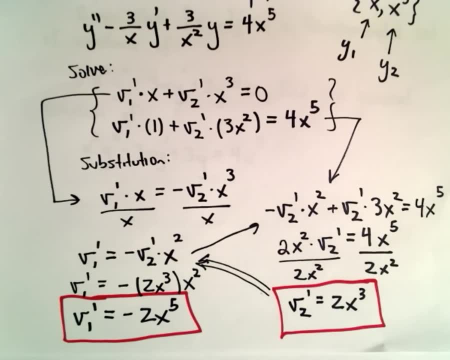 Sometimes you have to express your solution in terms of a definite integral, Which is okay. Sometimes that just simply happens, But this one is going to work out a little bit nicer for us, Alright, so let's calculate some antiderivatives. 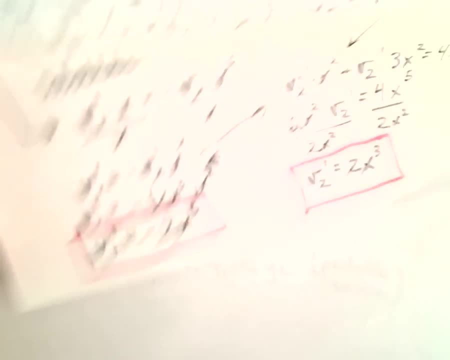 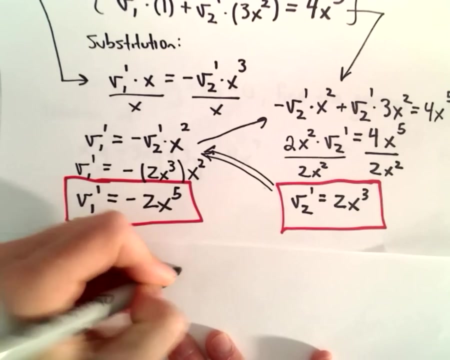 For these. you don't have to stick on the constants, You don't have to worry about that stuff. So let's see. So, v1 prime, that's negative 2x to the 5th. Well, if we compute an antiderivative, that's just simply going to give us negative 2x to the 6th. 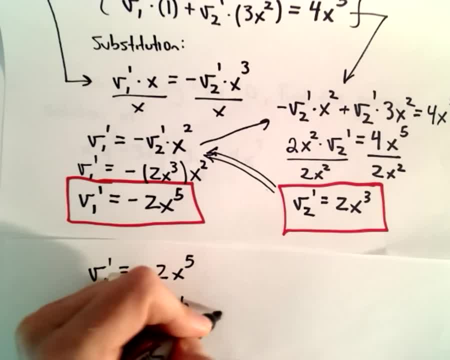 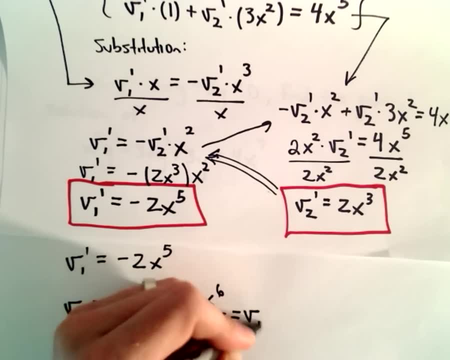 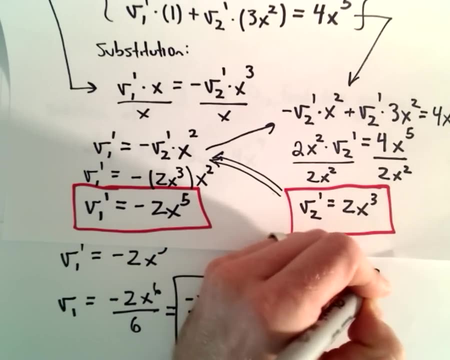 x to the 6th over 6,, which is going to be negative, x to the 6th over 3.. So that's going to be our function v1.. Same thing to calculate our v2.. So v2 prime is 2x to the 3rd power. 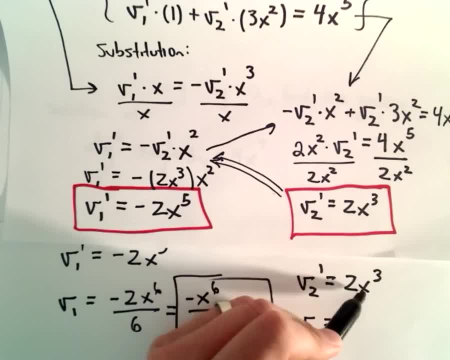 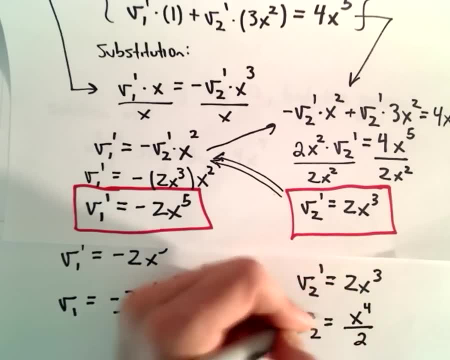 And if we simply calculate v2, we would get 2x to the 4th over 4.. So 2x to the 4th over 4 would just leave us with x to the 4th over 2.. 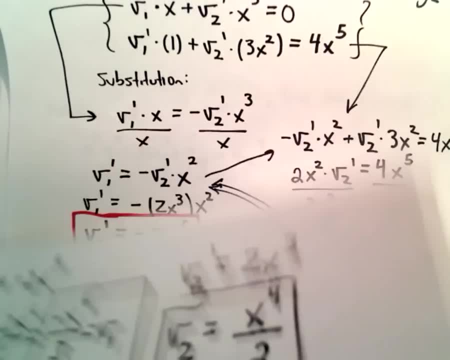 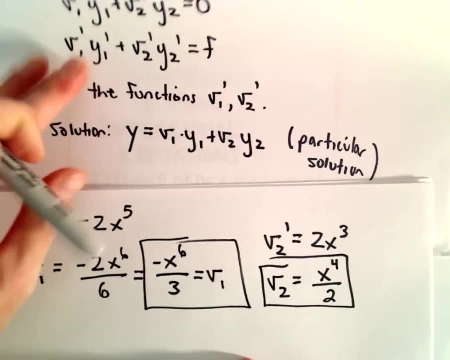 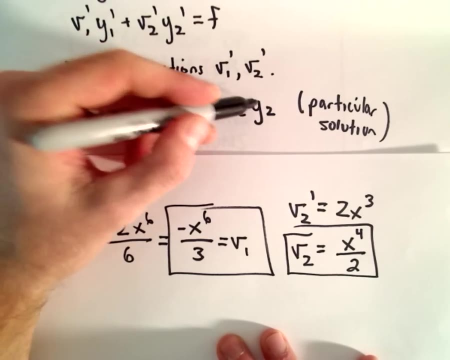 And now I'm just going to simply fill in my equation. We said: to get the particular solution, we said: to get our particular solution, we just use this equation: y equals v1 times y1 plus v2 times y2.. So that's what I'm going to do. 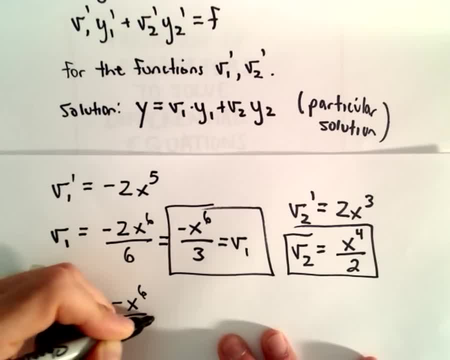 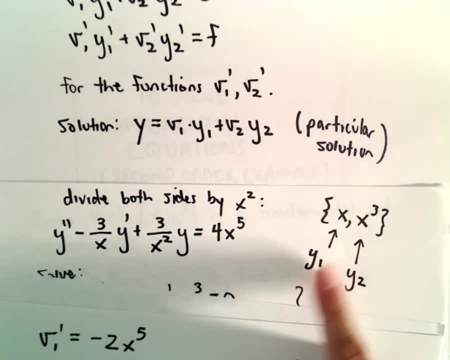 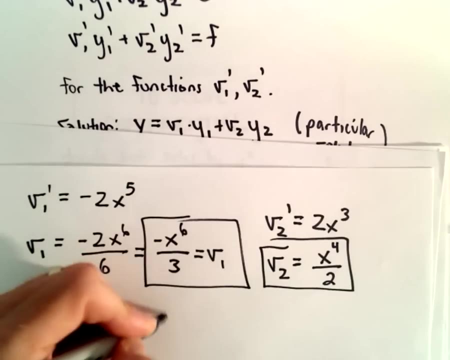 So v1, we said that's negative x to the 6th over 3.. Recall that our original y1, that was the first particular solution we had Which was, excuse me, one of the fundamental set of solutions. So we said y1 was equal to x plus v2, which is x to the 4th over 2.. 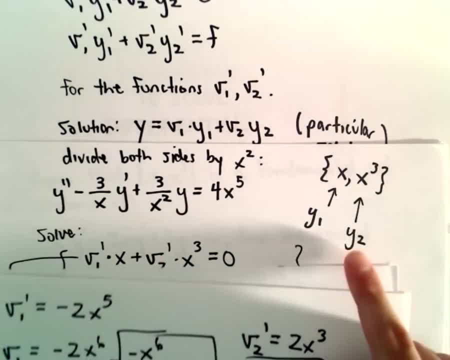 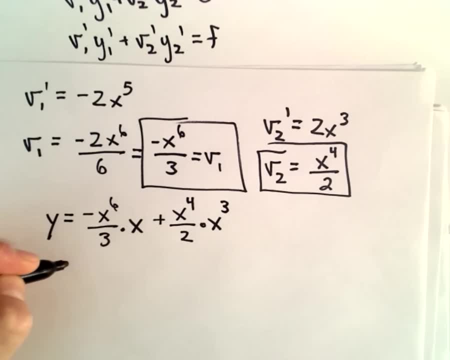 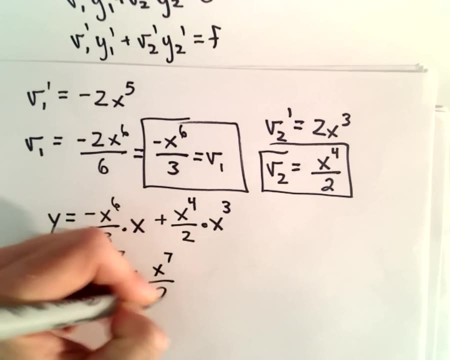 We multiply that by our other solution from our fundamental set, So y2 is equal to x to the 3rd, And let's see here: So I'm getting negative x to the 7th over 3 plus x to the 7th over 2.. 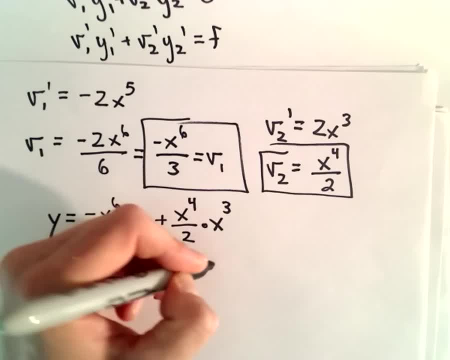 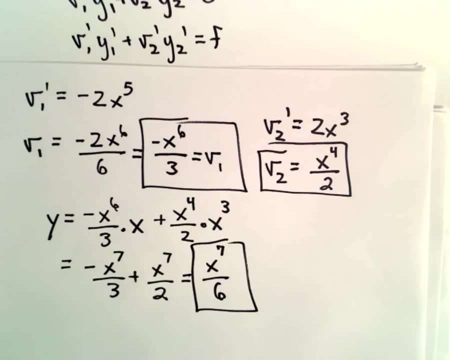 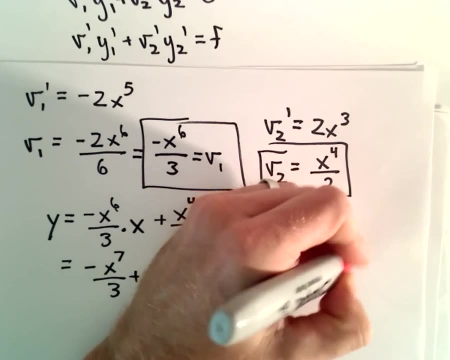 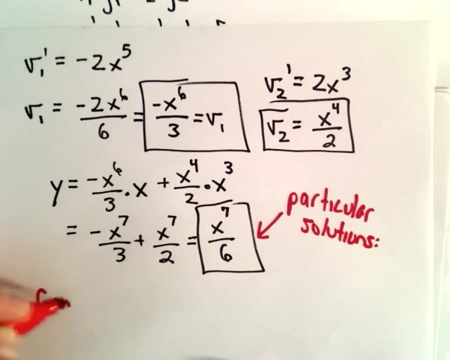 And you can check my arithmetic here: After I simplified, I got x to the 7th over 6.. Okay, so this is a particular solution, This is one of our particular solutions, And to get the general solution, all we do is we take our particular solution.